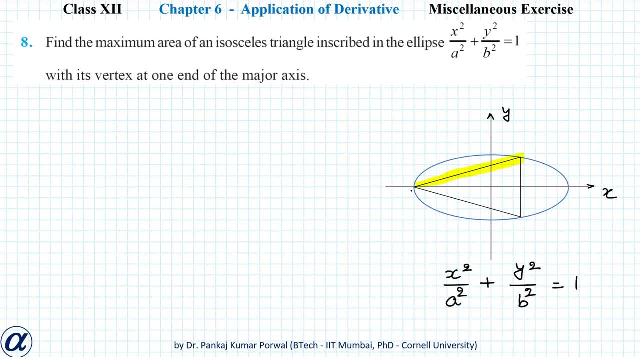 this is an isosceles triangle. the length of this side and this side will be equal and the x-axis will be angle bisector for this angle and that will be perpendicular to this side of the triangle. and these two vertices will be reflection of each other in the x-axis, So x coordinate. 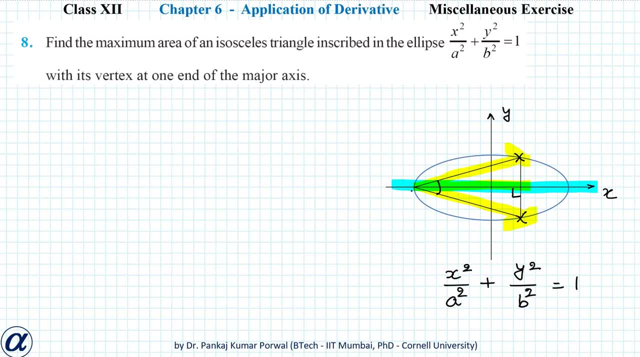 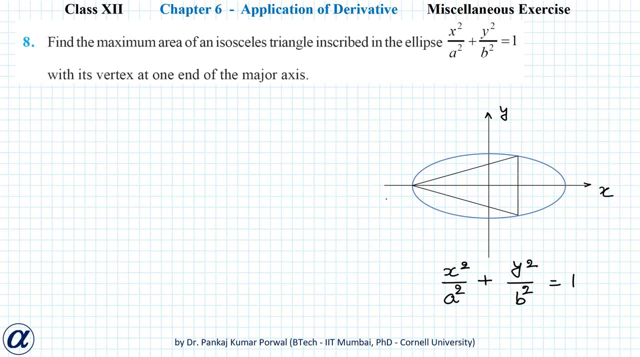 of these two vertices will be equal and y coordinate will be equal in magnitude, with opposite sign and the coordinates of ends of the major axis- This one be minus a comma 0. this one will be a comma 0, and coordinates of the points on the ellipse. 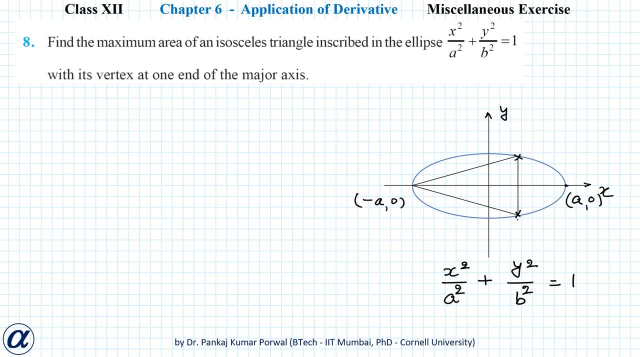 can be written either in terms of x and y or in parametric terms. if I write coordinates in parametric terms, then if this point I write is a cos theta, b sine theta, then the point right below that point will have coordinates a cos theta minus, b sine theta and the corresponding 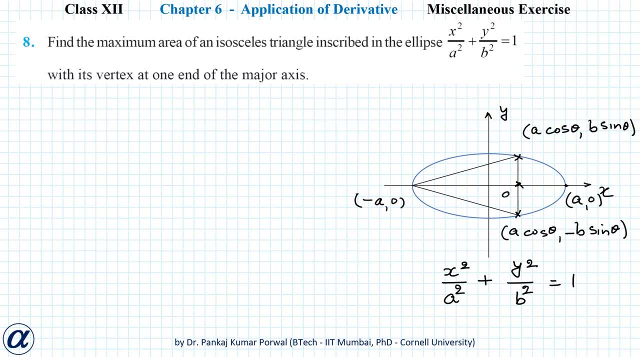 point on x axis will have coordinates: a cos theta comma 0. now we want to find the triangle which has maximum area, so let's write area of this triangle. area will be a cos theta equal to half base into height. the base will be this distance, ie distance between this. 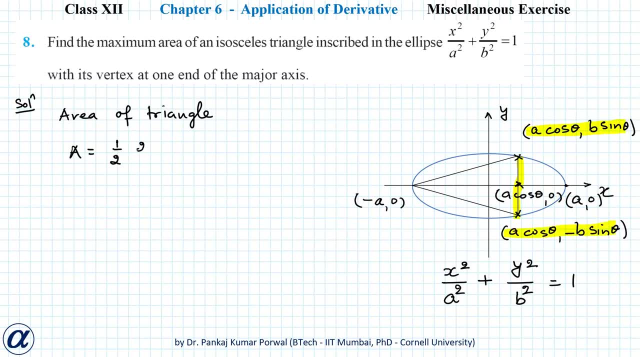 point and this point, and that will be 2b sine theta, because the x coordinate for these two points is same. so we just have to take absolute value of the difference between y coordinates and height will be this distance, the difference between these coordinates will be this distance. 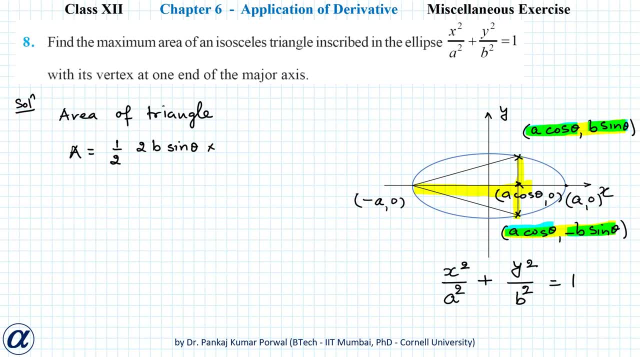 and again y coordinates will be actually height. all right, we write a bar as a dot. coordinates are same for these two endpoints. So we just need to take absolute value of difference between x coordinates of the points. So that will be a plus a cos theta, This I. 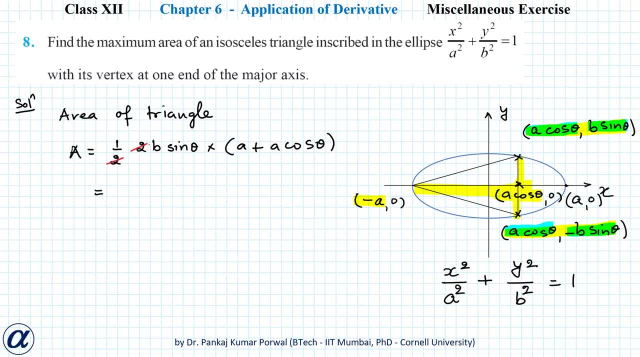 can simplify. So this 2 will cancel this 2 and I can take a common from this expression. So I am left with AB sine theta, 1 plus cos theta. That is my area of the triangle inscribed in the ellipse, And here the variable is theta, because for different values of theta I will 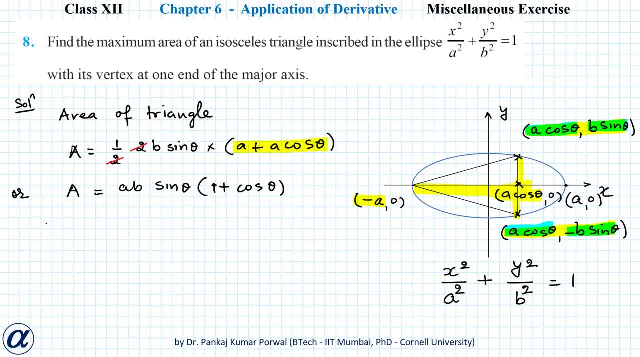 get different points on the ellipse. So to maximize A I need to do DA by d theta, which is equals to 0. so let's find dA by d theta first. so that will be AB cos theta. 1 plus cos theta plus sine theta into derivative of 1 will be 0, derivative of cos theta will be minus. 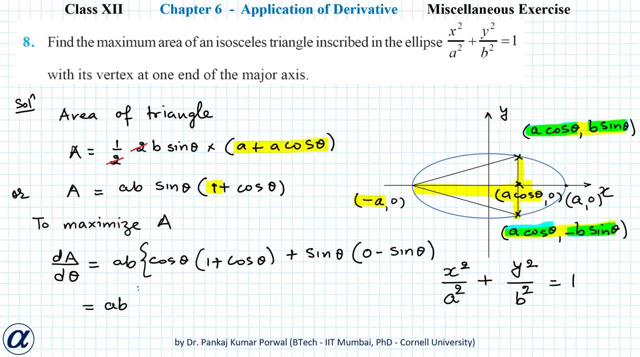 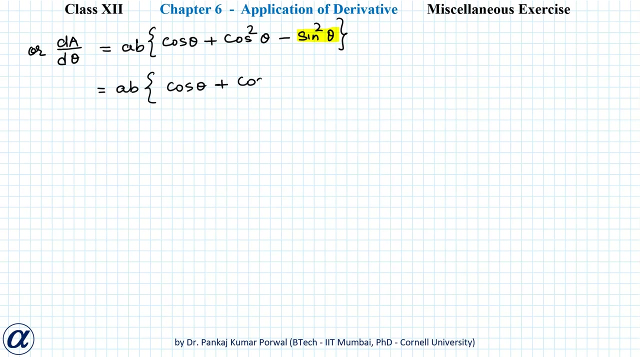 sine theta. so that is equals to AB cos theta plus cos squared theta minus sine squared theta. so this I can further simplify by writing: sine squared theta equals to 1 minus cos squared theta. so I get AB cos theta plus cos squared theta, minus 1 plus cos squared theta. this. 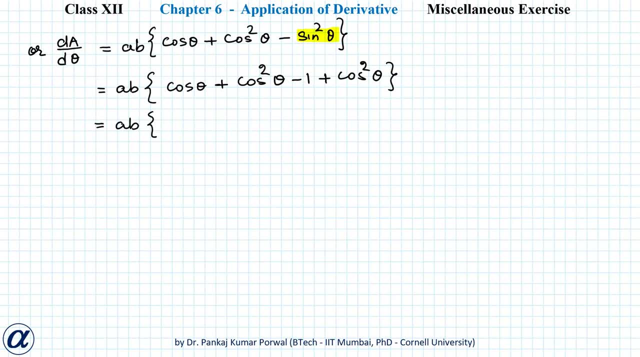 I can further simplify so that will be AB here. cos squared theta plus cos squared theta will be 2 cos squared theta plus cos theta, theta minus 1. now this expression is quadratic in cos theta, so I can factorize this by splitting the middle term so that will give me 2 cos squared theta plus 2 cos theta minus cos theta. 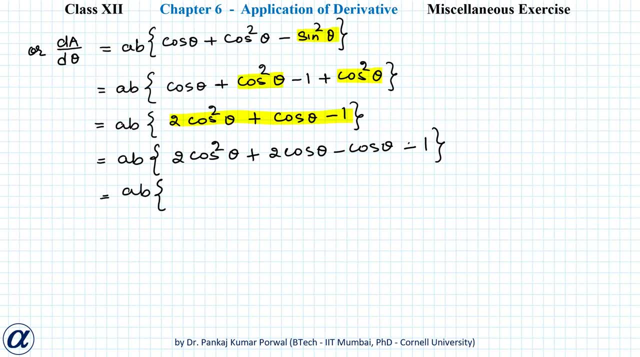 minus 1 equals to AB. from these two terms I can take 2 cos theta common, so I am left with cos theta plus 1.. from these two terms I can take minus 1 common, so that gives me cos theta plus 1, that is. 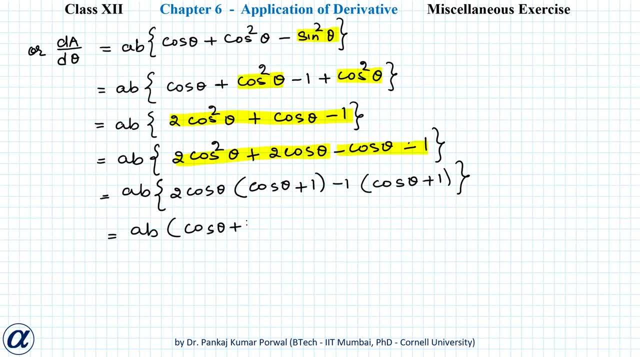 equals to AB, cos theta plus 1, to cos theta minus 1, and if I set this equals to 0. so that gives me cos theta equals to minus 1, cos theta equals to 1 half, and corresponding to these two solutions, I can find values of sine theta also. so sine theta when cos theta. 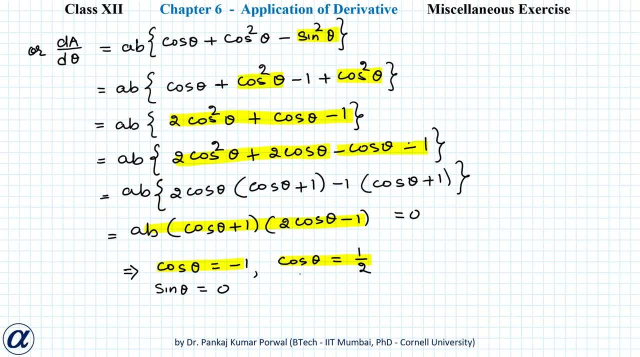 is minus 1 will be 0, and when cos theta is half sine theta is root 3 by 2. this we can find by using formula: sine theta equals to square root 1 minus cos squared theta. now to find at which value of theta we have maximum, we will have to do. 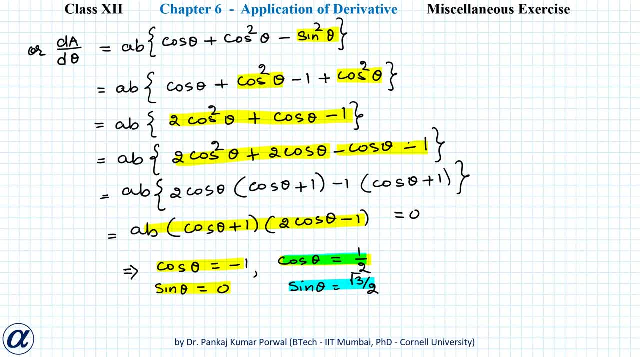 second derivative test. for that I will have to find second derivative of A that I can find by differentiating dA by d theta and for that I will use this expression so this expression can be differentiate as d2A by d theta. 2 will be equals to AB minus 4 cos. 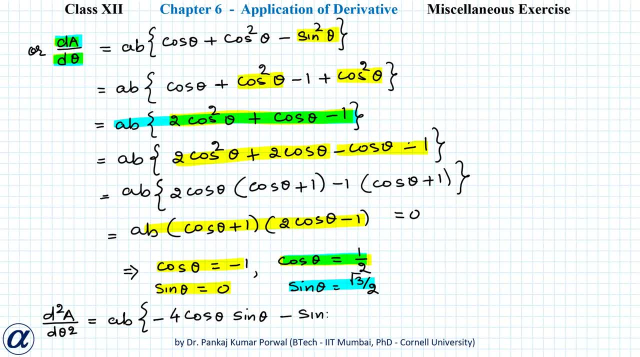 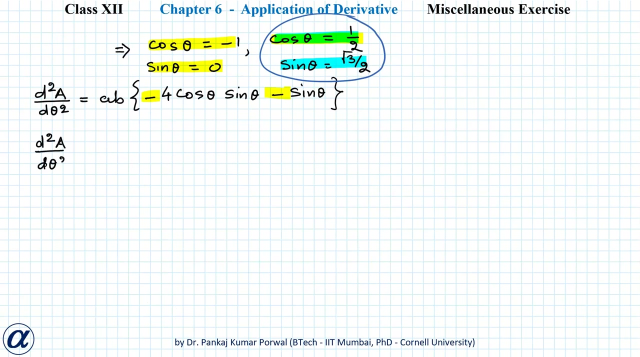 theta sine theta, minus sine theta, derivative test derivative of minus 1 will be 0. so because there are minus signs in both terms, so I will first check second derivative of A about this point: theta. so d2A by d, theta 2 at cos theta. 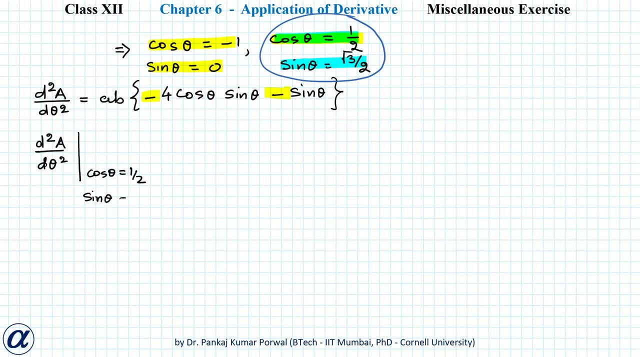 equals to half and sine theta equals to root 3 by 2 will be equals to 0.. derivative of minus 1 will be equals to AB minus 4 into 1 by 2, into root 3 by 2, minus root 3 by 2. this clearly is negative. so we have maximum when. so to find maximum area. 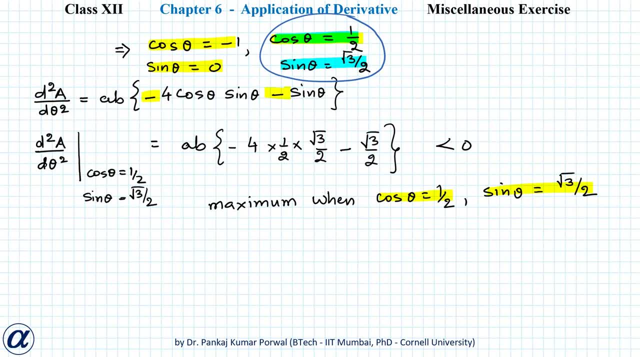